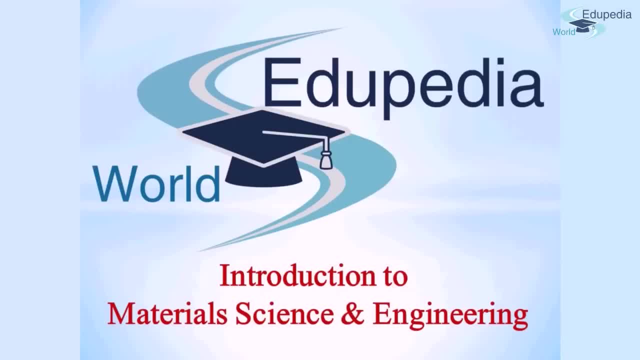 Hi, thank you for joining us again. Welcome back to the course on Introduction to Material Science and Engineering offered by Edupedia World. Previous several lectures we have been understanding the idea about crystal systems and we saw the different type of crystal systems that exist both in the metallic world and in the ceramic scenario. 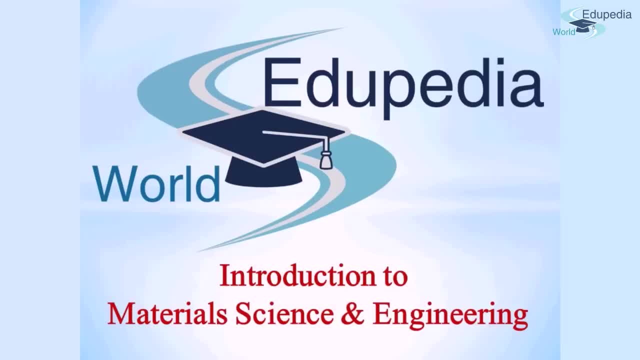 Today we will jump into one very important concept that is important in context of crystalline materials. We will be understanding the idea of crystallographic directions and crystallographic plane. Today's lecture, we will be focusing on crystallographic direction, but before that, let us introduce you to the idea that why do we need to understand crystallographic directions and planes, and what exactly are they? 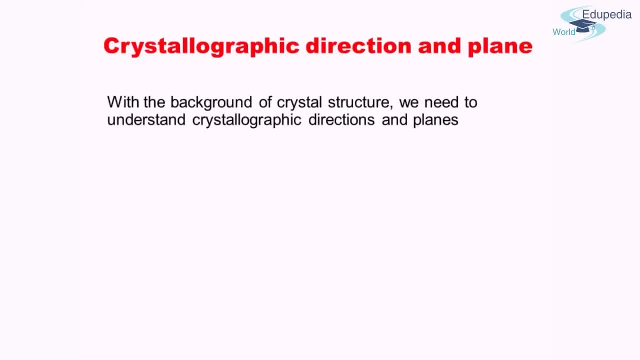 So, as I said, with the background of crystal structure, Now we are ready to understand the crystallographic directions and planes. but why do we need to understand it? The reason is quite simple. The reason is that the deformation, or any deformation which takes place in a metal or a ceramic, takes place in certain directions and in certain planes. 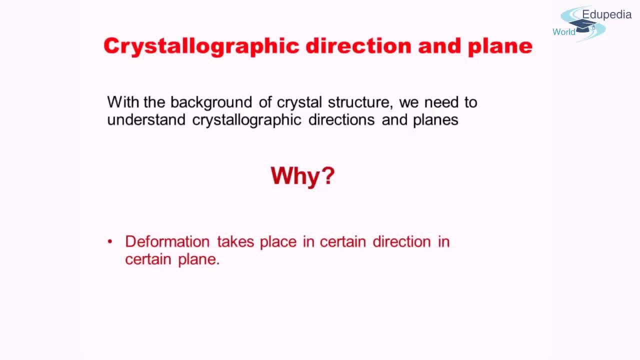 So we need to know which are the directions and planes which are favorable for deformation And thereby we can understand, And thereby we can identify those planes and directions and follow the phenomena and understand the physics behind it. Secondly, there are several material properties, like conductivity or elastic modulus for different materials, which can vary with directions or which can vary with the crystal orientation. 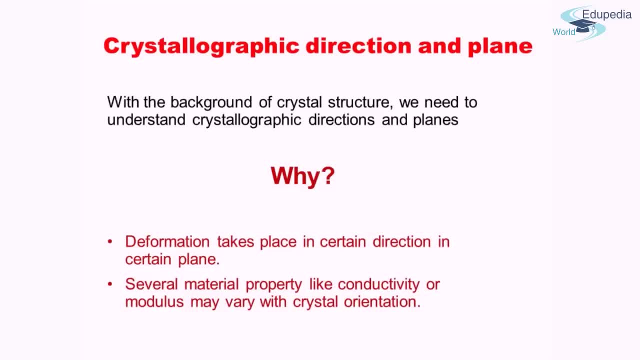 The orientation with the crystal is existing. So in order to understand those physical phenomena, We need to have a background of the crystallographic directions and plane. Therefore, we need to understand both these concepts To begin with. today's lecture will focus on crystallographic directions. 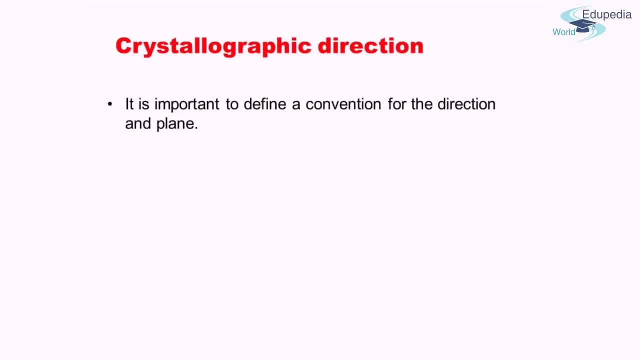 So what is so important about crystallographic direction? As I already mentioned, we need to understand it, to understand the basic physics behind different kind of deformation and stuff. There is a need to establish a convention. There is a need to establish a convention. 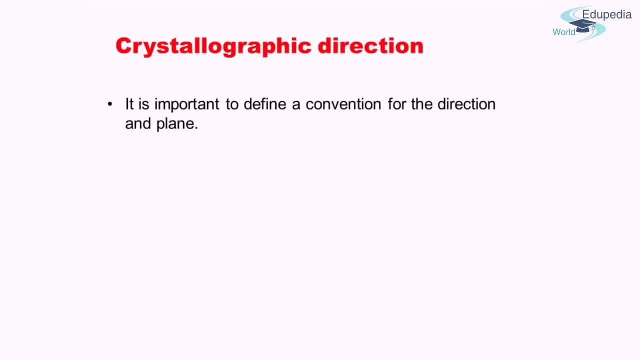 There is a need to establish a convention Beforehand to understand both crystallographic direction and plane. That is, everyone who studies material science or metallurgy should use a unique set of ideas to represent a particular direction. There should not be any confusion. 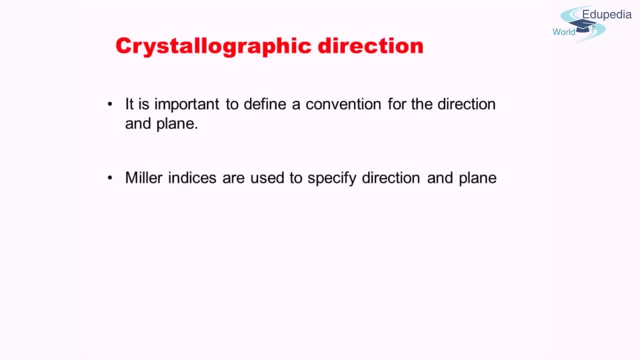 Therefore, a convention needs to be established. The convention that is used is known as Miller indices. Okay, And this Miller indices is used to define specific direction And specific plane. How do we do that? We will see further down the line. The idea is that any unit cell which you have seen till now, 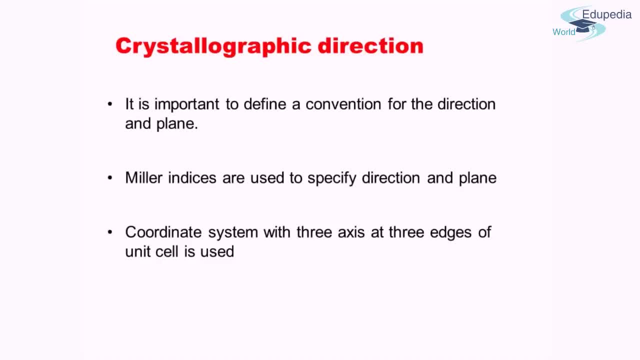 The cubic unit cell, for example, Can be defined by three axes: The x-axis, the y-axis and the z-axis, Right Or the z-axis. So we use those three different directions As the three edges of a coordinate system which we define. 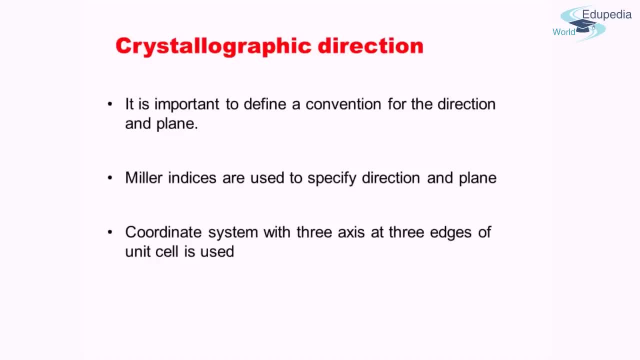 And based on that coordinate system, we define the crystallographic direction. First of all, I will give you a theoretical idea about what or how we are going to do it, And then I will practically show you, with figures and examples, How do we define direction. 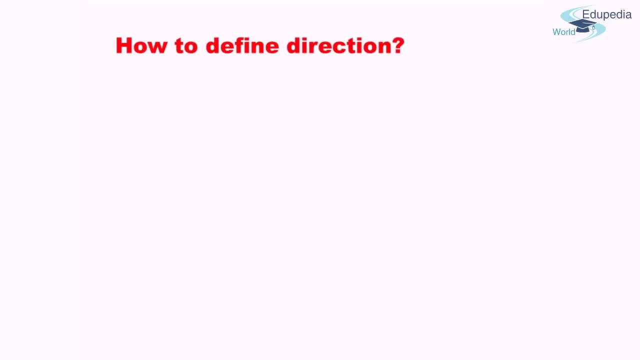 In general as well as in this specific case of crystallographic direction. So for any direction, imagine you want to establish the direct direction from your home to your home. So your home is one point, Your school is another point And you draw a line from your home directly towards your school. 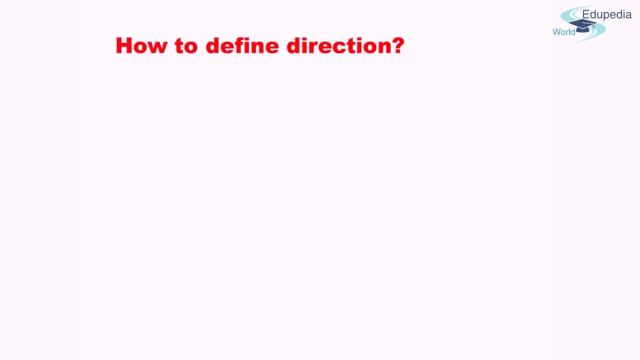 That gives you a direction That may be north, northeast or 15.5 degrees south of east, Something like that. Right, So you have a specific direction using the convention of south east, northwest. Similarly, here what we use is that for crystallographic direction. 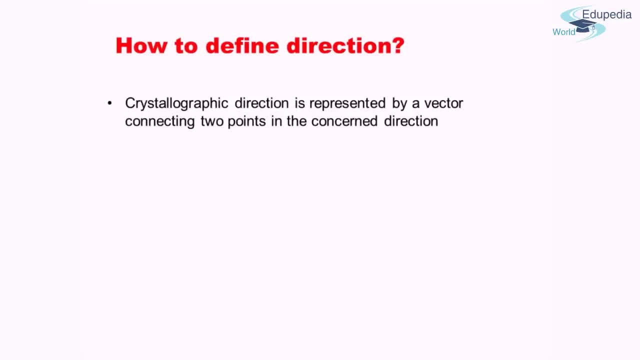 We use the vector representation. And by vector representation what I mean- It's parallel to the example of school and home which I just gave- Is that we connect two points in the concerned direction And then what we do is this vector which we have got. 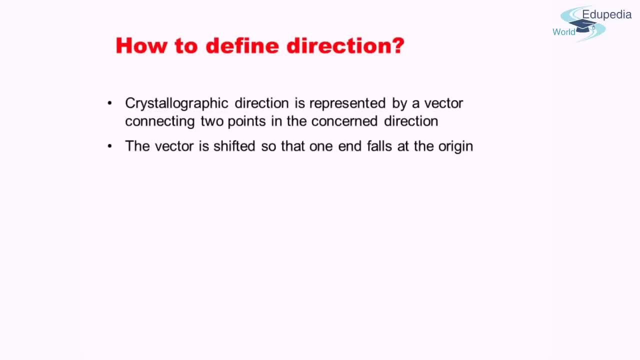 We shift it such that one end falls. The starting point falls at the origin. Okay, Now we have one end at the origin of the unit cell And the other end is pointing towards any specific direction. Now that end will kind of help us define that direction of the whole direction. 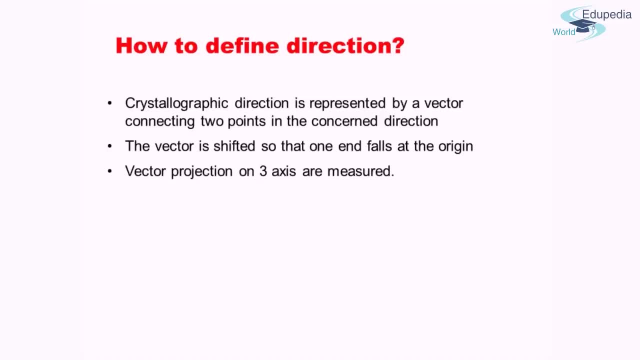 So what we do is that now we vector project that vector on three axis And then we measure the length imparted by the vector projection on each of the three axis. Stay with me, I'll show you it practically. Then they are reduced to the smallest integral ratio. 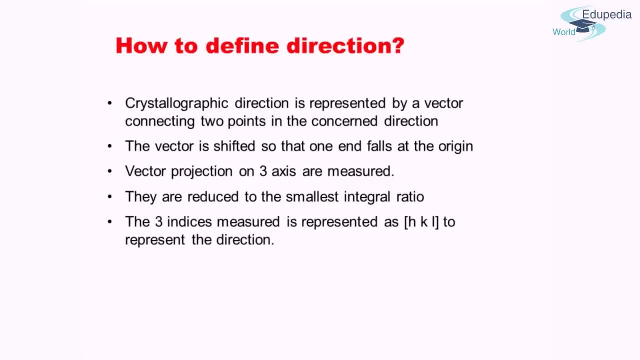 The three indices which we got by the vector projection are then represented as h, k and l. in this kind of bracket You need to use the square bracket to represent the direction, And important point here is this square bracket is used for a single direction. 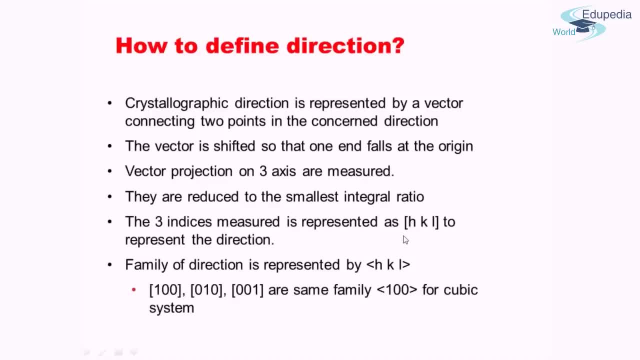 But we, if we have a family of direction- I'll come to what a family of direction is- But if we have a family of direction, we can represent it by this curve bracket with h, k, l, The Braville indices mentioned inside the curve bracket. 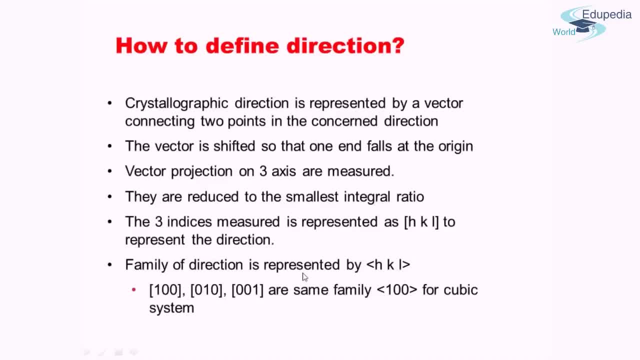 Now, what is the family of direction? A family of direction refers to all the directions which has, which can be expressed like this: For example, a family of direction for one zero zero is the direction of the curve. A family of direction is the direction: one zero, zero, zero, one zero and zero zero one. 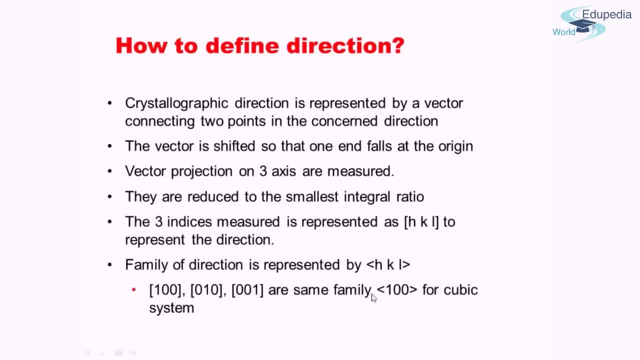 Okay, for the cubic system. So this gives you an algorithm of the step-by-step definition of how to find that direction- crystallographic direction- But I'm quite certain this does not give you any insight about how exactly to do it. So let me try to show you roughly over here and explain what I meant by each of them. 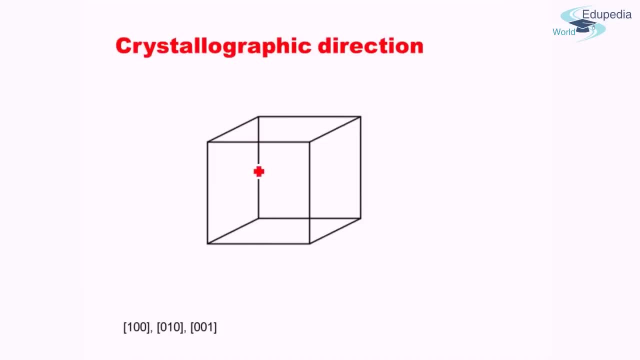 Let's do it in the next page. So here I already have a cube. We will be discussing about the cubic system for the time being, And what we do is that we first establish our coordinate system. I normally use this as my x axis, y axis and z axis. 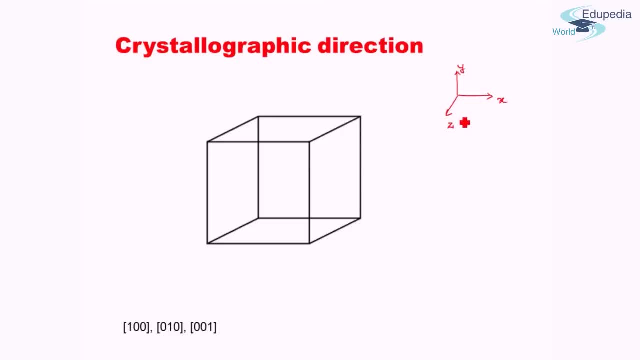 Remember that the axis selection should always be such that it follows the cross rule, That is, x, cross y should be pointing towards the z axis. Okay, the cross product rule should not be valid, invalid. So this is the convention I will use. 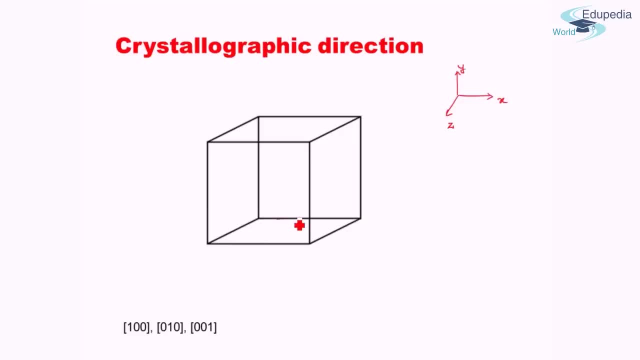 Therefore, this direction is the, this direction is the x axis, This is y axis and this is the z axis. Therefore, when we what we find out that this is the origin right, This point is the origin of the unit set. Now suppose you are saying: 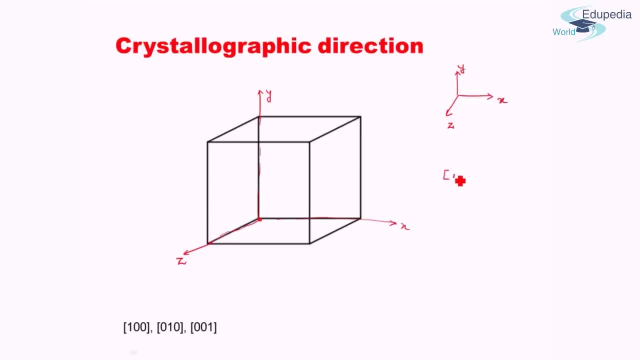 That you need to find the direction. one zero zero, one zero zero. So how do you find out the direction is that you take one step towards the x axis along the x axis. So one step along the x axis will be from here till here, right? 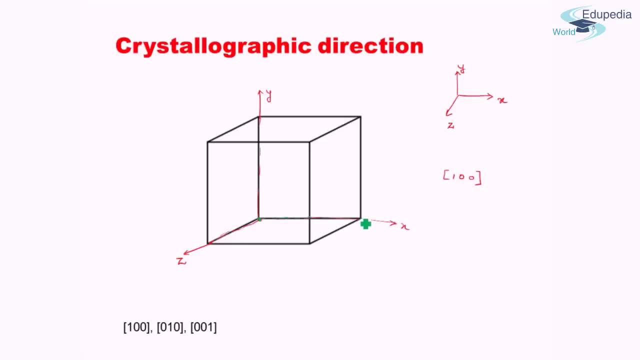 So we start from here and we are at present over here. Then, y axis: we take zero steps, So the arrow remains here. Z axis: we take zero steps, So the arrow stays over here. Therefore, one zero, zero direction is given by this axis. 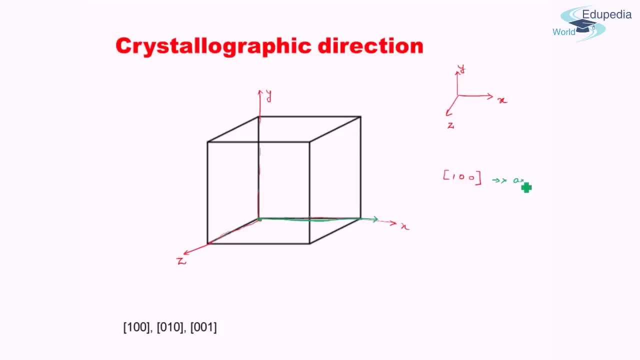 So this, in fact, is the x axis itself. So one zero, zero direction is this direction. Similarly, if you want to find out the zero, one zero direction, How do we do that Zero in the x direction? So it remains at the origin. 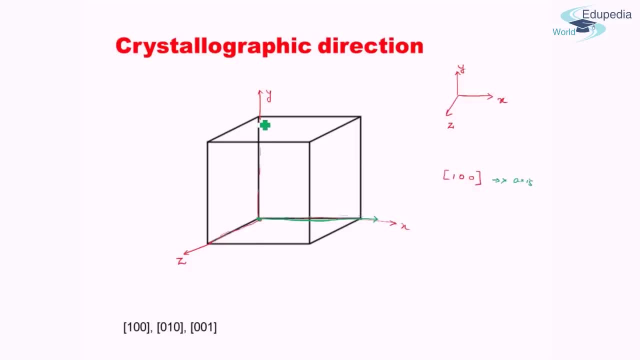 One in the y direction Goes till here, Zero in the z direction, So it remains here, Thereby zero. one zero is nothing but the y axis. Okay, So this is zero, one zero. This was one zero, zero by similar logic extension. 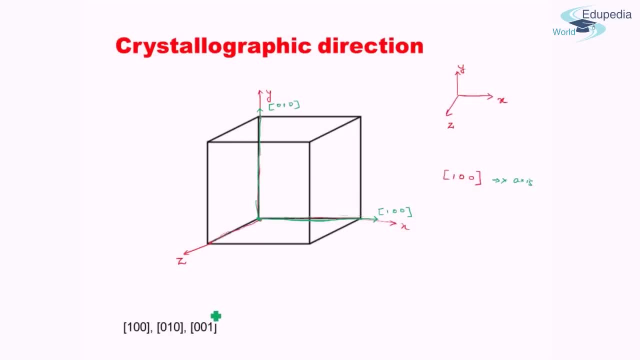 Zero, zero, one will be zero step in x axis direction, Zero step in y direction and one step in z direction. So we have the zero, zero one. So this is zero, one zero instead of one zero. So we have zero, one, zero. Zero one zero is nothing but the z axis in this direction. 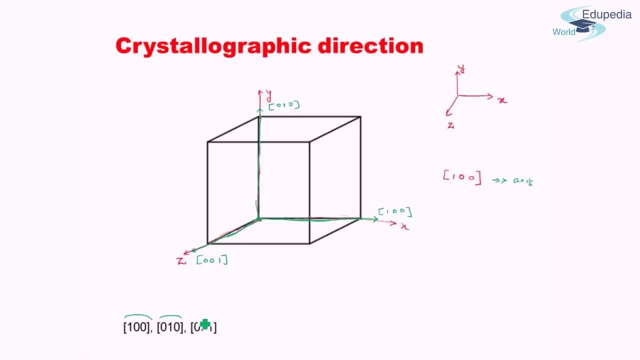 Right Now. this was an example where we already had the Bravais lattice Miller indices. This where the Miller indices Right And using that Miller indices we find, found out what is the direction of that Miller indices. Now let us say that the Miller indices is not given, but the direction is given. 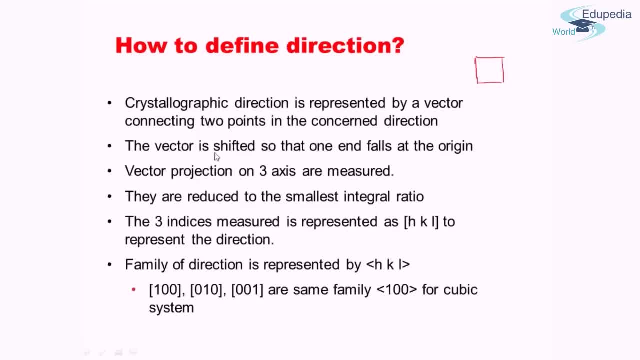 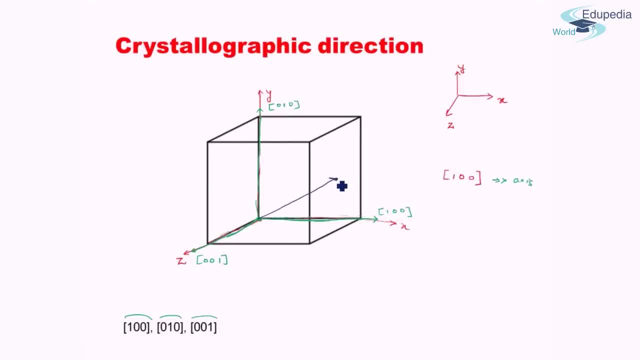 And you are asked to find out the Miller indices. That is where algorithm, which i have shown here, will be used. so let me do that. let's say, let's say we have to find the direction of miller indices, of this direction, now let me define it for you, this length. 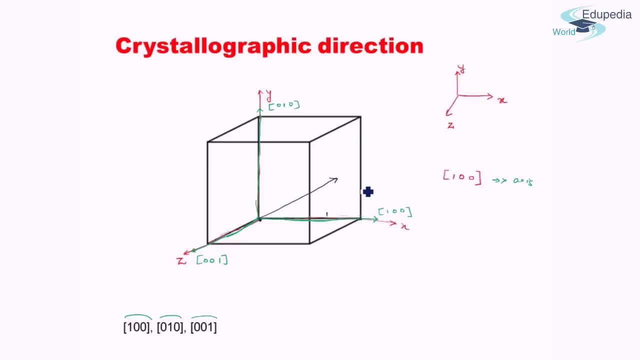 is one unit. okay, then this length, this much in the y direction is half unit, and this length, or this length in the z direction is also half unit. so what we have done is to move in this direction. we have actually moved one unit in the x-axis direction, a half unit in the y-axis. 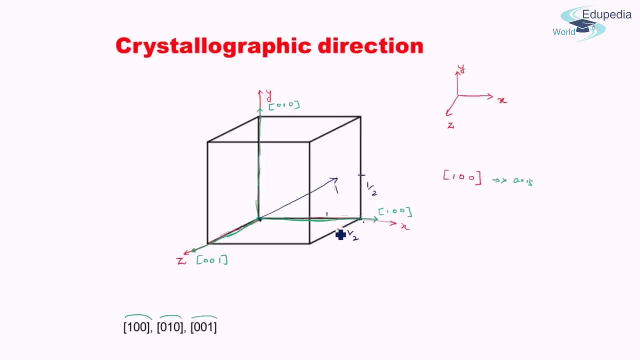 direction and half unit in the z-axis direction. thereby we have got this line. therefore, what will be the miller index for this line? this line miller indices will be one in x-axis, half in y-axis and half in z-axis, but, as i have said, in the algorithm that 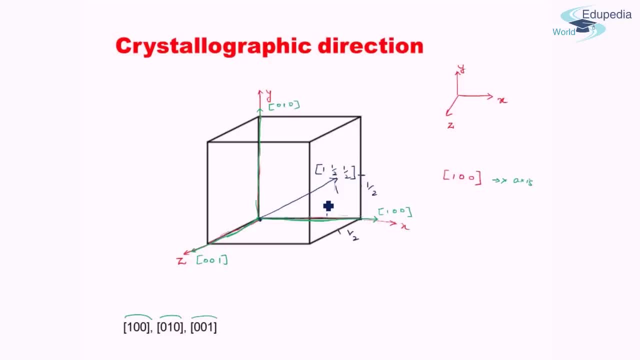 and this is a matter of fact or a convention. yeah, this is a matter of convention that we do not keep fractional miller indices. we do not keep fractional mirror indices in crystallographic direction. so what we will do is one half half needs to be converted to the nearest integer. how can we do? 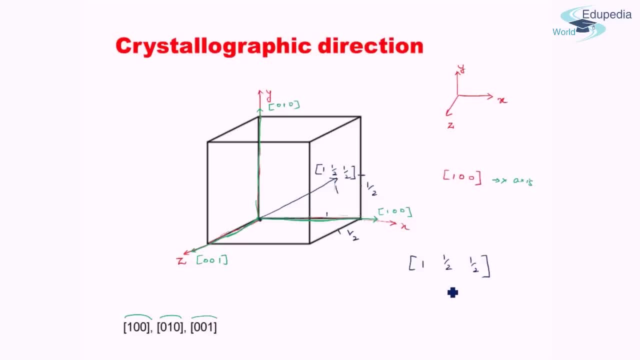 that we can do that by multiplying it with such a number that all the fractions get converted into a integer. so if you multiply all the three indices by two, so if you multiply it by two, then what we get? we get one, two, one, one. and now i make a claim that this direction and 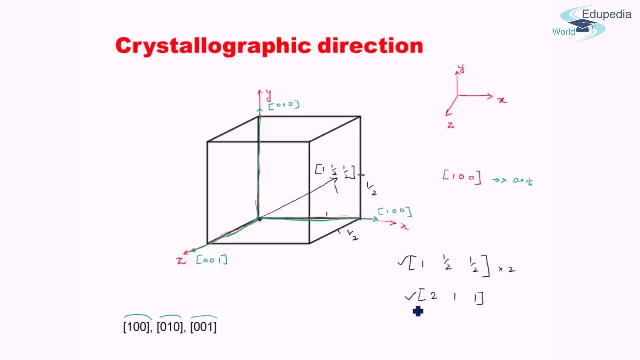 this direction are the same direction. okay, fair enough, i have made a claim, but how do we verify this? how do we say that this and this direction are the same direction? let's see, let's try to figure out. what is this direction? two one one. so, for two, one one. what we need to do is we need to 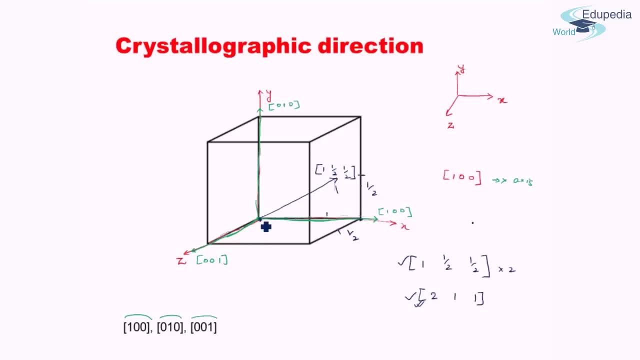 go one step, two step in the x-axis direction. so i have gone two step in the x-axis direction, one step in the y direction, so i go from here till here, and then one step in the z direction. so basically, i come in the z direction one step. thereby, what you will get is, ultimately: 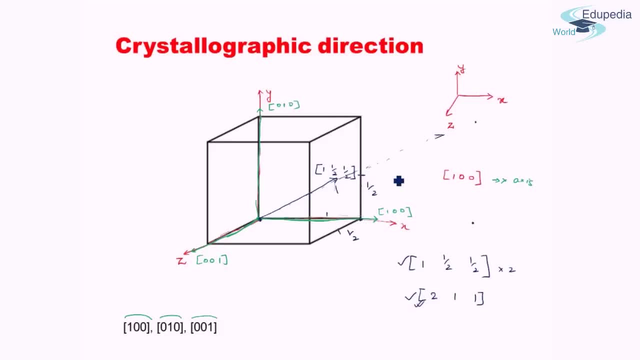 you will get something like this. okay, so this will be something which will be two, one one. i'm certain it's a bit confusing here, because this is a 3d projection which i'm trying to draw in two dimension, but take my word for it or you can. 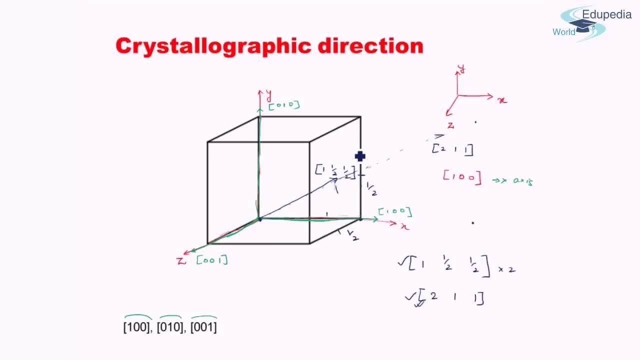 actually draw two cubes here right, one cube and one cube of the same dimension over here too, and then you try two steps in x-axis, one step in y-axis and one step in z-axis and see that it will be the same line but extended, and just twice the length of this line. 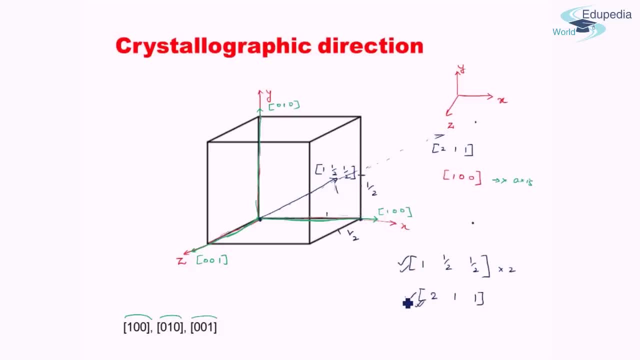 thereby my claim that this direction and this direction are same is a valid claim. okay, so you can say: i can express this also as 4, 2, 2. obviously you can do that, but as a matter of convention, what we do is we keep it to the smallest integer. okay, so this gives you an idea about if you have a 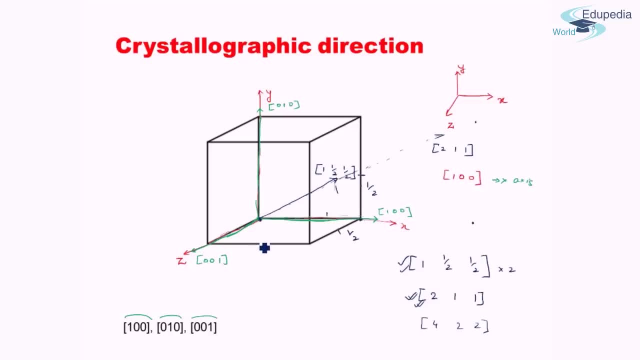 miller. if you have miller indices given, how to draw the direction out of it. or if you have the direction, given the arrow drawn, then how to find out the miller indices out of it. right, let us use some more practice here. let's try to figure out what will be 1, 1, 1 direction. so for one, one, one. 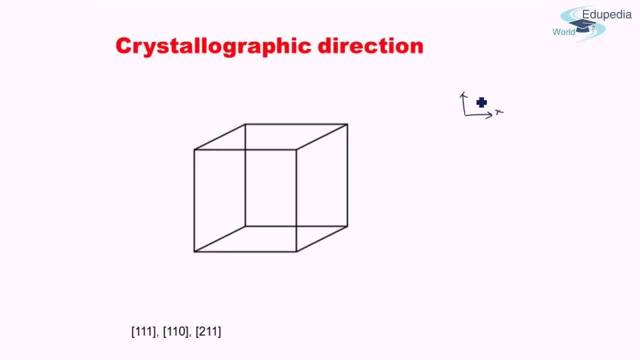 direction, what we'll do again. my convention will be same: x, y and z-axis. so i take one step. this is my origin. i step, take one step in the x direction, then one step in the y direction, then one step in the z direction. i reach over here. so my initial position was here, final position is here. so the 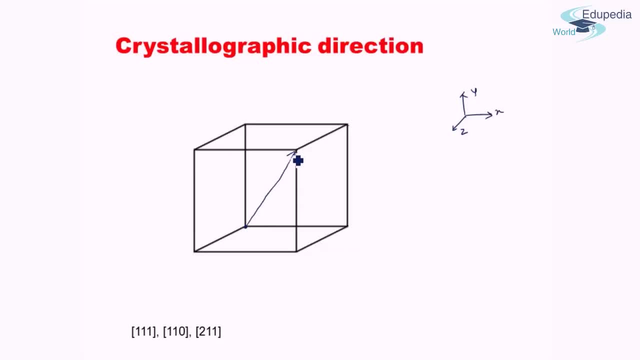 direction. one one one is basically this direction. okay, this is one one one. now let us try out one one zero. one one, zero. again the same thing. it's a simple exercise. you just need to keep your convention intact and follow the number of steps provided here. so, one step in x-axis, one step in. 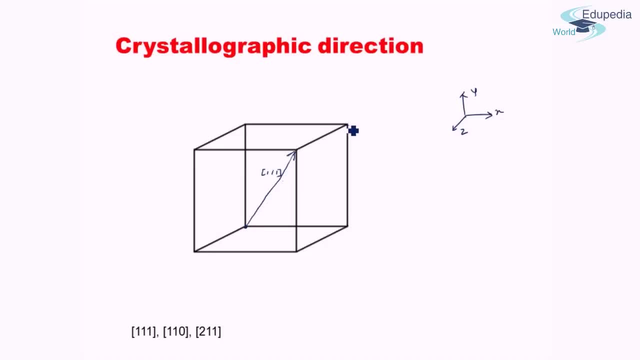 y-axis, zero step in z-axis. so it ends over here, starts from here. therefore, it will be like this: this should obviously be a straight line: one one, zero. now, uh, let me bring an interesting example: two one, one. how do i draw? two one one, two one one means i take two step in the x-axis. so i go from: 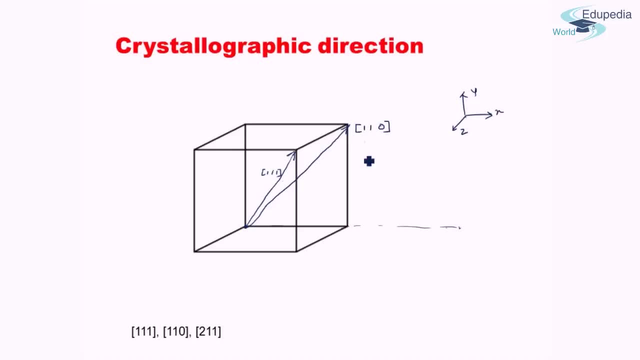 here to here. okay, till here. let me actually draw another cube, okay, so that you can visualize it easily. so this is roughly my second cube, which is of the same size as this cube, and now i want to go two step in the x-axis. so this is one step, this is two step i have. 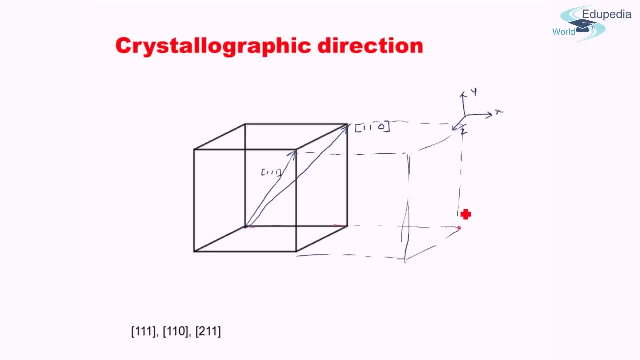 raised here. then i go one step in the y-axis- i have raised here- and one step in the z-axis, so ultimately i end up here, starting from here. so the two one one will be basically this direction. okay, if we go back one step, this is the same two one one which i tried to draw in this slide, right? 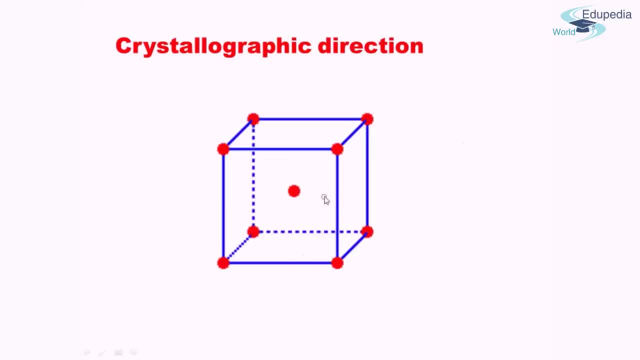 so you can see that the two one one is actually passing through. sorry is actually passing through that point i talked about. it is passing through this point. so here we have verified our claim in the previous slide. okay, now let's draw a few more lines and try to figure out what are the crystallographic direction for those lines. 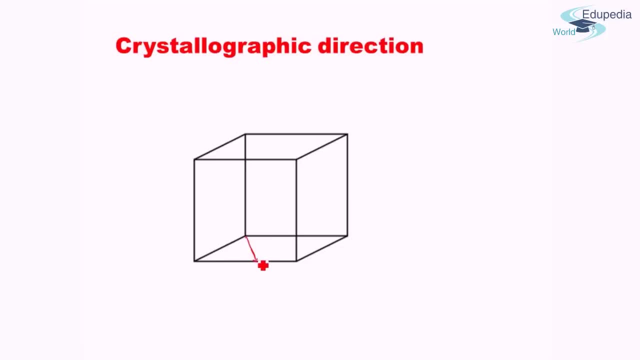 in the cubic system. let's say i have, i have this direction, what will be the miller indices for this direction? and i am using the same convention, the x-axis, y-axis and z-axis, and i say that this is again half the length, one by two, okay. so how can i get from here to here what i need to do? 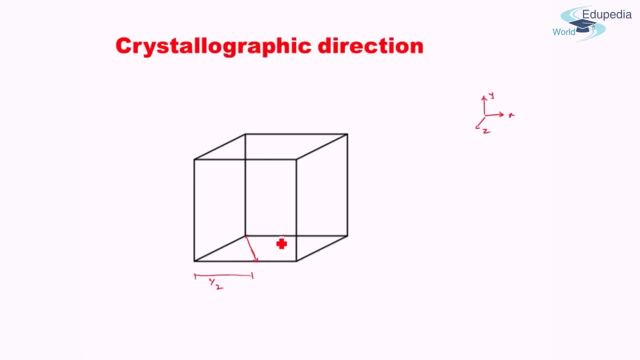 is i need to traverse half length in x direction. this is half x and one complete length in y direction. right, one complete length in y direction and in z direction. i don't need to go anywhere. so what is happening is i went half x, one y and zero z. now, multiplying it by two, i get one to zero. 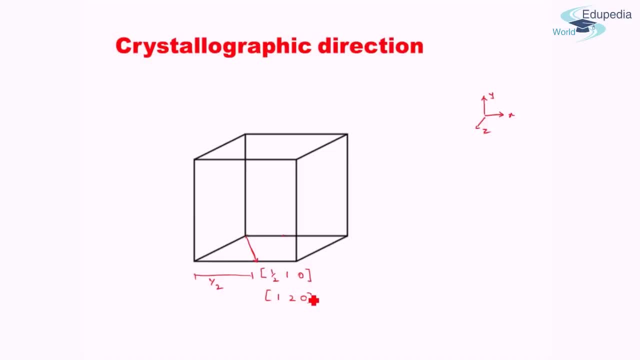 so this is one, two zero direction. one thing which i forgot to mention is while writing down the direction in the miller indices format, there should not be any any commas here. it is read as one, two zero and it is written the same. now suppose i have something. 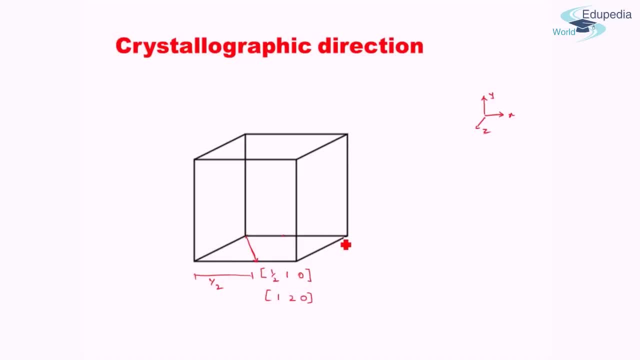 let's do something a bit tricky. okay, let's do the starting point here and the ending point here, okay, so now the direction which i have is not starting at the origin, rather it is over here and it goes till here. so what i can do is either i can shift this vector. 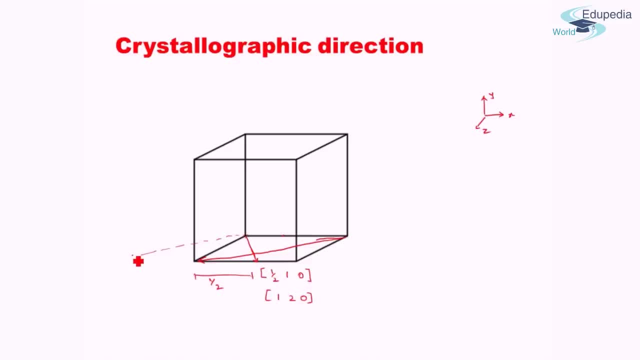 parallel to itself and bring it over here. right, or what i can do? i can redefine the axis as, or redefine the origin as the origin to be here rather than there. okay, so let's do it by redefining the origin. this i am taking as origin now: zero, zero, one, zero, zero, zero, rather so. 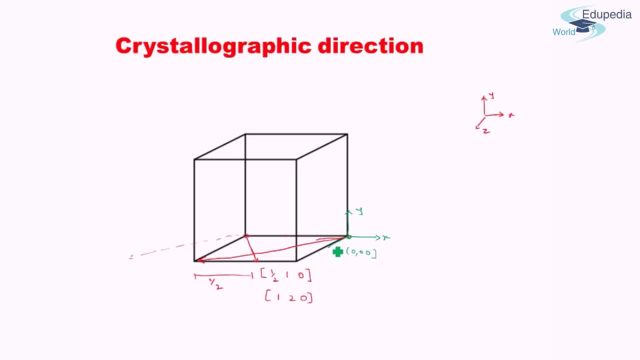 let me draw it out: x, y and this is z. so what is happening? how do i get from origin till here? what i need to do is i need to take one step in x direction, but in the negative direction of x, right? so let me first write it down: negative: 1 in x direction. 1, 0 unit in y direction. okay, 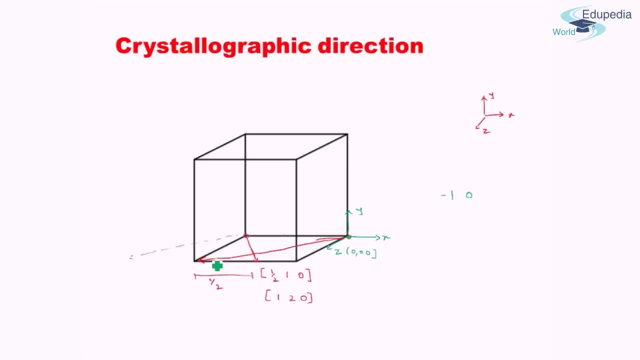 0 in y and 1 in z, 1 in z, 1 in z. so this is my direction for this vector, which is z minus 1, 0, 1 c 0 in x direction minus 1, 1 in x direction. one c 0 in j direction minus 1, but in the crystallographic 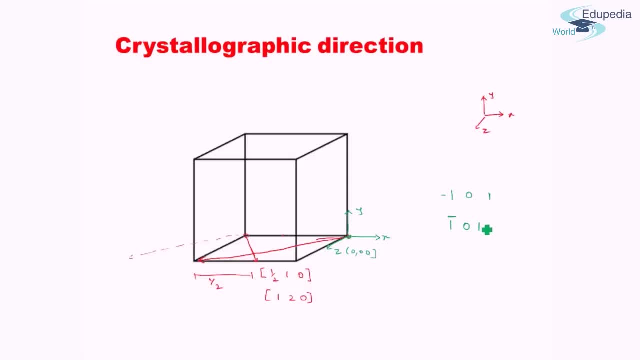 direction reference. we do not use minus one, rather we write it as bar 1, bar 1, 0, 1. so this direction is bar one, zero one. fine, i made one mistake over here is that i said one step in the y direction. actually, there is zero step in the y direction and one step in the z. 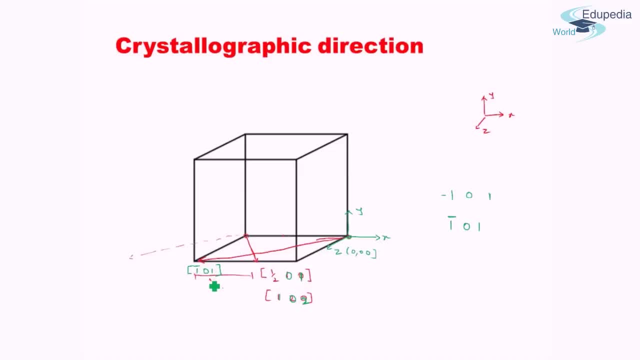 direction, so it should be 1, 0, 2- pardon me for that- one step galleries: zero, zero, zero, zero. that fine. coming back to this, what i have pointed out is that you might have negative braville indices, miller indices, right. so if you have negative miller index, what you do is you write. 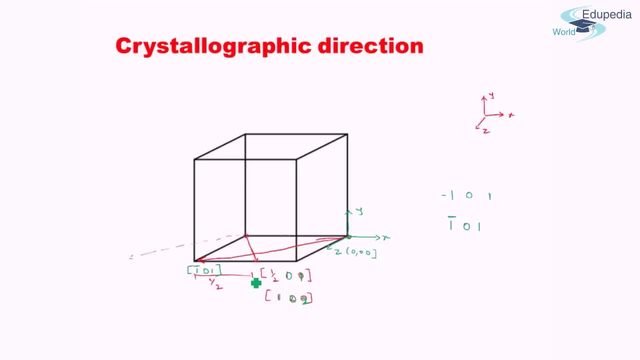 it. represent it by a bar instead of a minus sign before. that is the convention. okay, let's close with one more example. let's say: let's say, if we have something like this and this direction is 1 by 3, now, since we are starting from here again, i am putting the origin here. 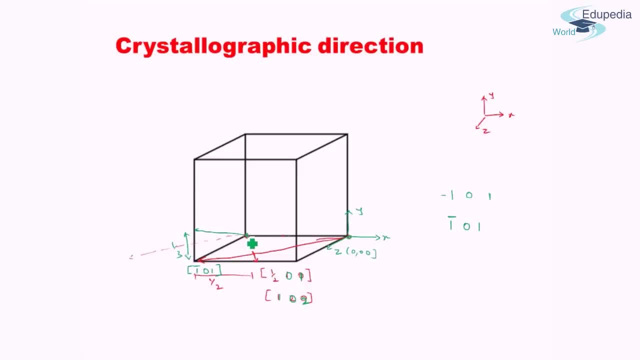 i am going in: x direction, 0 units, y direction is 1 by third unit and z direction is 1 unit. so it will be 0, y direction, 1 by 3 and z direction, 1. and this i rewrite it as 0, 1, 3. 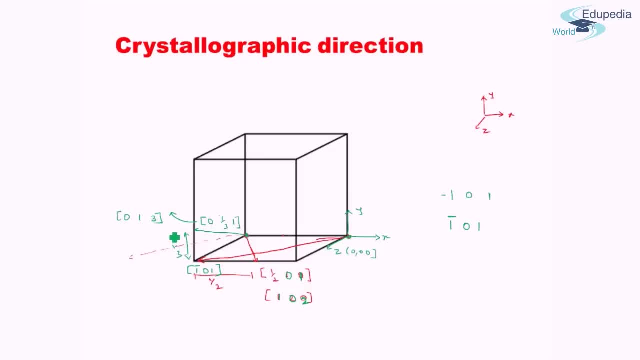 by multiplying by 3 so as to get the smallest integer at each place. now, this must have given you a good grip about how to find crystallographic directions. and in case of cubic systems, let us see example of body centered and face centered in the body centered example as, if you remember correctly, we know that the diagonal 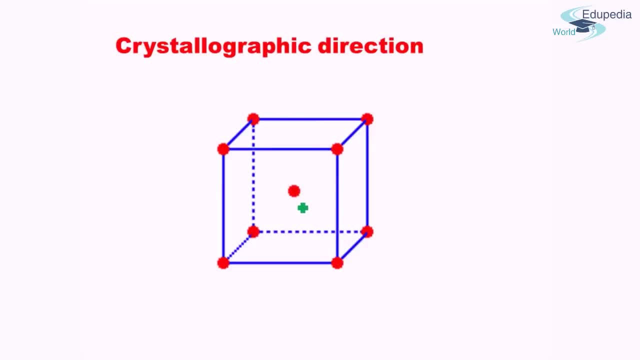 the body diagonal is the diagonal along which the atoms are touching each other. so let's find out that miller indices for the body diagonal. what is the body diagonal? this is the body diagonal right passing from from the body, coming from this end to this end again x, y, z. so what is happening? 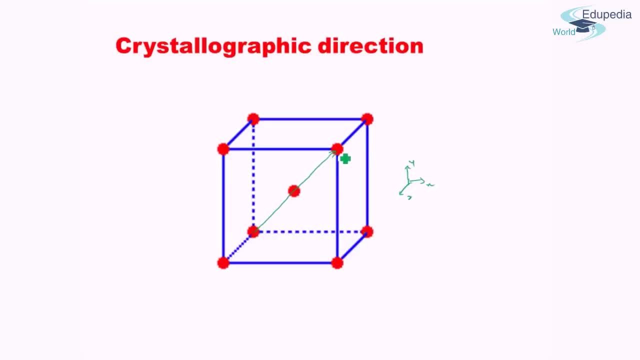 one step in x direction, one step in y direction, one step in z direction. so the body diagonal is one one one. so our closed packed direction for a body centered, cubic, is one one one. this is quite important which will utilize while studying deformation. so closed pack for bcc is one one. 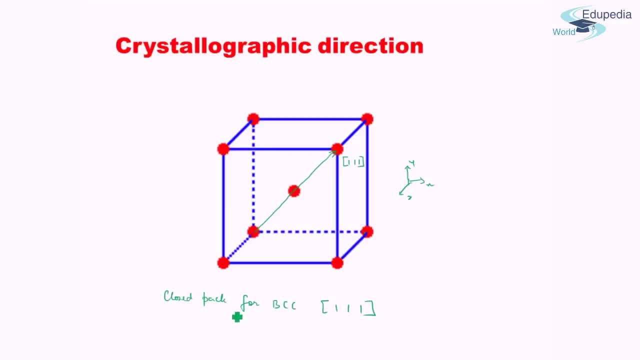 one direction. why is it called closed pack? it is called closed pack because that is the direction in which the atoms are touching each other. now for a face centered cubic. if you remember, we had the atoms touching each other along the face diagonal. so what is the face diagonal? the?